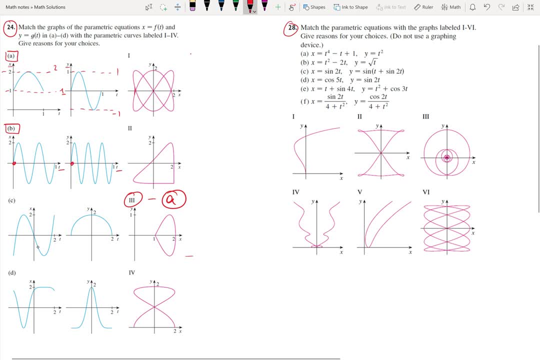 So we can see: this is my x is t, and when t equals to 0,, what is my x and y component? in this case, Corresponding to the graph, my x and y are going to be 0, 0. So I know that my graph is going to intersect an origin at some point. 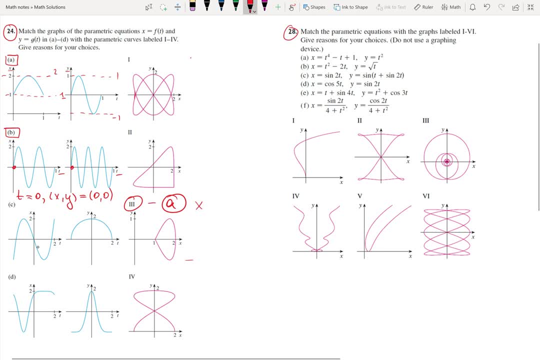 Third one. we don't need to check because we already know this is part a. but you can see in, third one doesn't work because it doesn't intersect an origin. Number 2 also doesn't work because it doesn't intersect the origin. 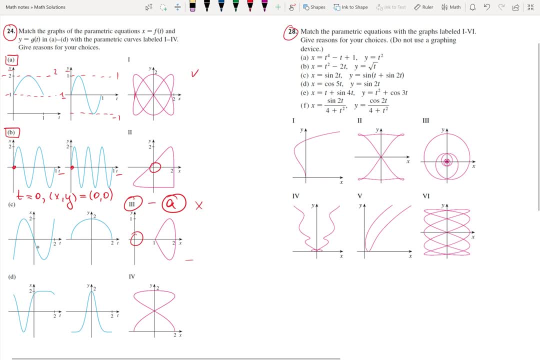 Number 1 is possible candidate, but number 4 also doesn't work, so this is going to be actual number 1.. So my 1 is going to be b. Okay, let's do the next one. c, and for c, what we can do. we can analyze how many maximums, and how many minimums do we have? 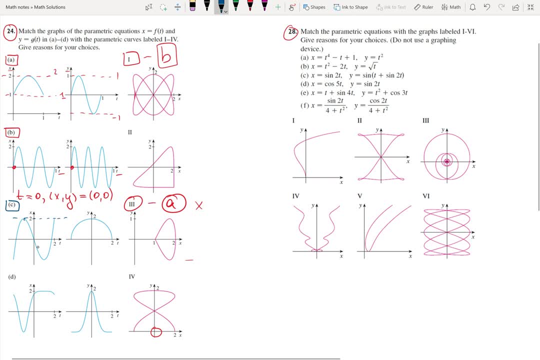 What does it mean? You can see over here that x has, for two values of t, two maximums over here, and over here let's say a and b, And for all intervals, For all t from minus 2 to 2, for y variable, we have only one maximum, c. 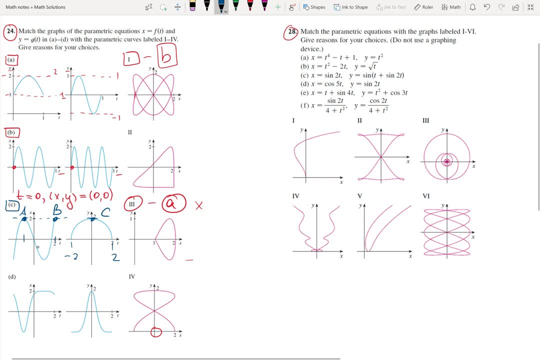 Let's take a look at the first graph. In my x direction I have two maximums over here and over here, So x is a possible candidate. but in my y direction I have three maximums over here, So graph number 1 doesn't work. 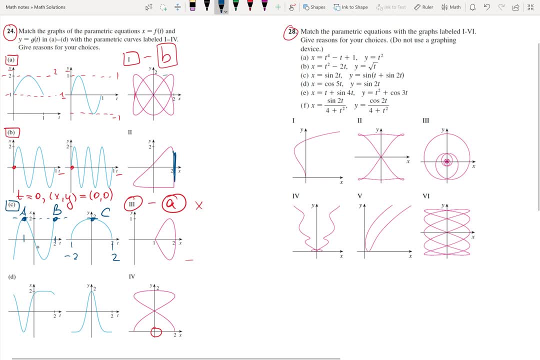 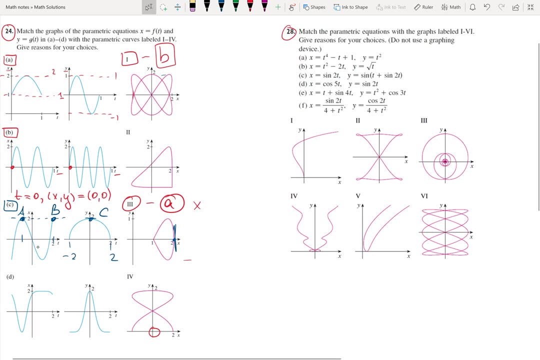 Graph. number 2 also doesn't work, because for x I have infinite, I have infinite many maximums, so we can skip it. For number 3 also doesn't work, because we have only one x maximum here, but corresponding to graph we should have a and b. 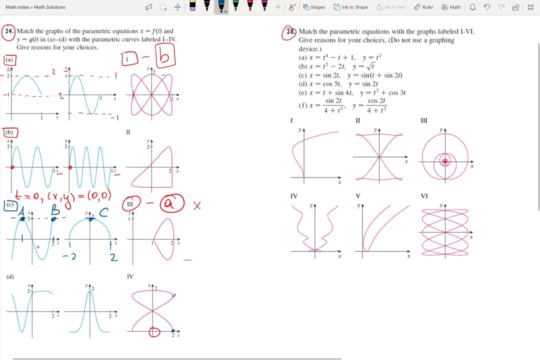 But for number 4, we can see we have two maximums in x direction and only one maximum in y direction. So this is going to be, for example, my- I don't know- like a, b and c. So from here I can conclude that number 4 is my c. 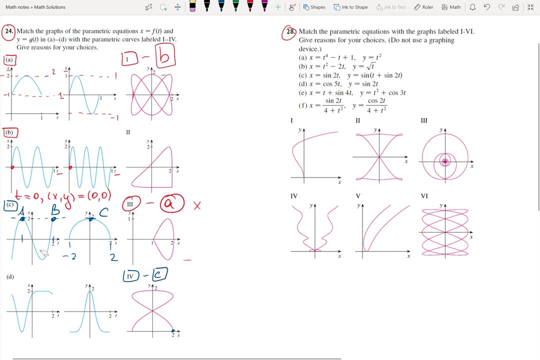 Okay, and let's analyze the last parametric equations graphs for number d. For number d, as we guessed, we can see it's going to be number 2.. So 2 is d, But let's find the way, the pattern. 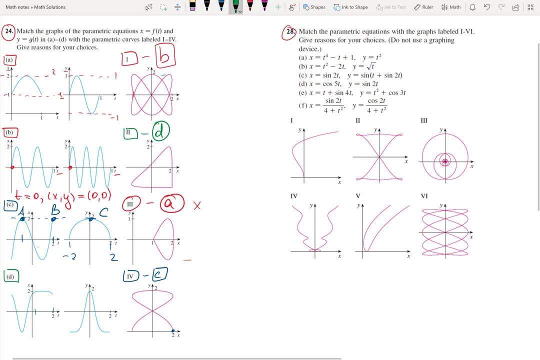 For example, in my x, I can see when t changes from a really small variable of t up to 2, my x is going to be constant, And this is exactly what corresponds on my graph over here. When t changes from like I don't know, like 0.005 to 2, my x is going to be constant, and you can see on this graph. 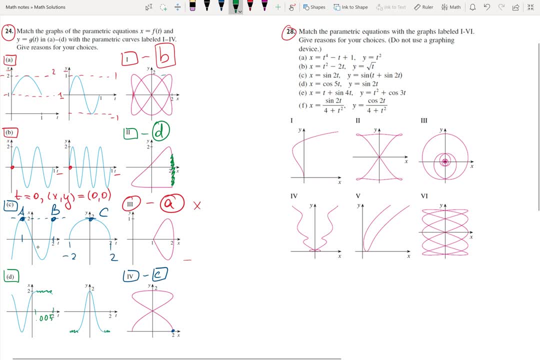 And the same true for y. When t changes from one variable, my y is pretty constant, So in this case I can see it's going to be corresponding to this part of my graph. Okay, so for problem 24, I'll show you different techniques, how you can recognize Cartesian graph based on parametric one. 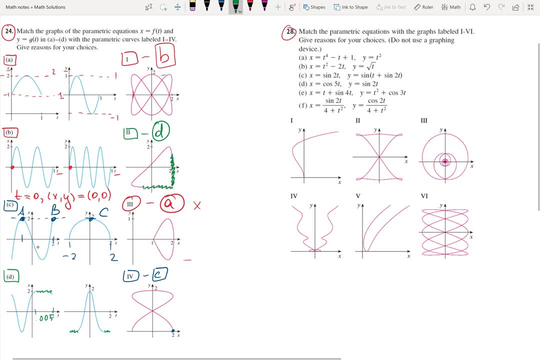 But let's move on to the problem 28. When my graph is going to be way more extreme and very more interesting. Okay, if you're going to take a look of each of this function, you're going to be scared Because, like this function, are impossible to graph. 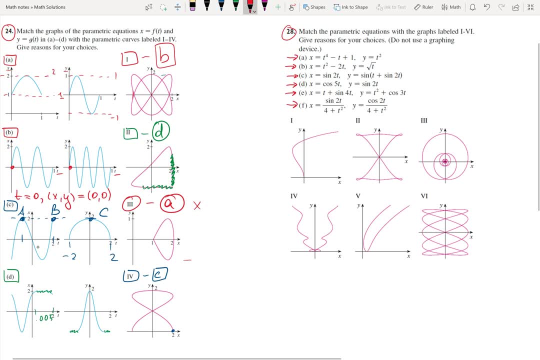 But I'm going to show you one of the example: how we can analyze this function and how we can find the corresponding Cartesian graph. Okay, I would like to start with function f. And for function f, I know: x equals sine 2t over 4 plus t squared, and y equals cosine 2t 4 plus t squared. 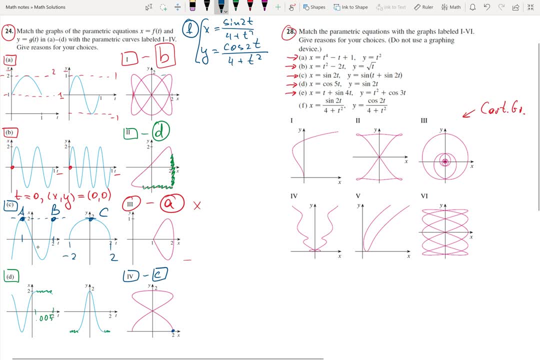 So let's take a look at this function. At first, we have no idea what this function looks like. Like, if you will try to eliminate the parameter, it will not work because, like it's just, this function is hard. 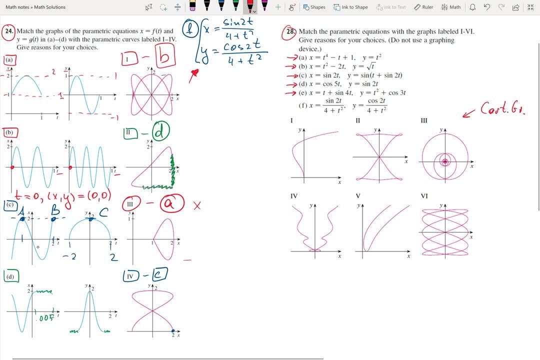 So, as soon as you see some hard problem or some hard function, the first thing that you should do you should find the way how you can simplify this function. I can see if I will cancel out 4 plus t squared. if I will just simplify it, I will just pretend there is no 4 plus t squared. 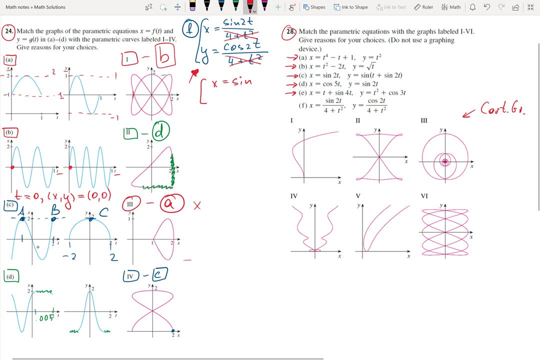 Then my function is going to be just x equals sine 2t and y equals cosine 2t, And for this one I know that corresponding Cartesian graph is going to be: x squared plus y squared equals to 1, because sine squared plus cosine squared equals to 1.. 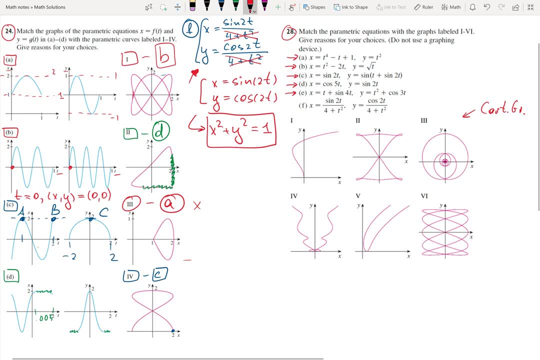 And then, since I know that approximate shape of my graph is going to be a circle in this case, I'm trying to come back to return my 4 plus t, squared for each case, And then I can see if I will take my bottom part. 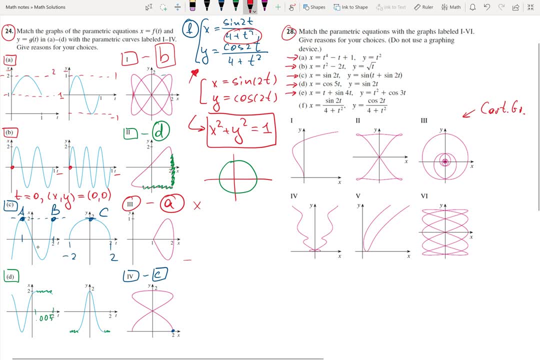 So approximate is the shape of my graph. It's going to be a circle, but when t increases my bottom will become bigger and bigger. So it means that my radius of my circle will become smaller and smaller, because my radius will be dependent on t. 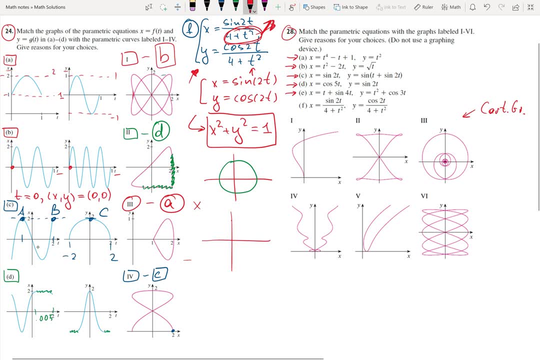 So what I will get if I will start to draw my circle. I will start with a big one, small one, small one, small one, something like this. And then I can take a look at my graph And what do I have over here? 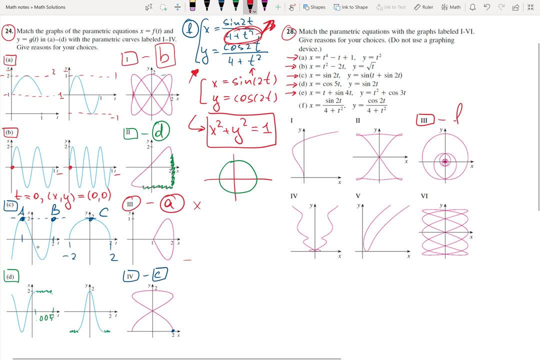 I have that. number 3 is exactly corresponding. It corresponds to the graph f, because I have bigger circle, smaller, smaller, smaller, And I can see that graph number 1,, 2,, 4,, 5, 6, it doesn't work. 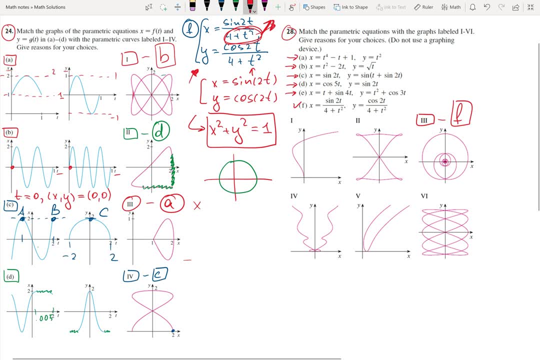 Okay, so number f is checked. Okay, what is the next easy function that we can do? Let's take a look at problem number e. For e, I can see I have x t plus sine 4t and y t squared plus cosine 3t. 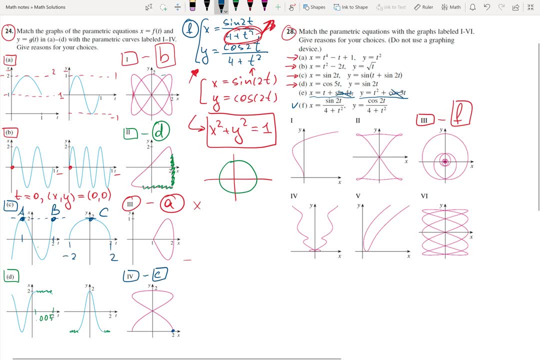 So what can I do? over here I can see that I don't have trigonometric functions And then my function is x equals t and y equals t squared. So from here I will have that y equals x squared. So approximately my function will look like a parabola. 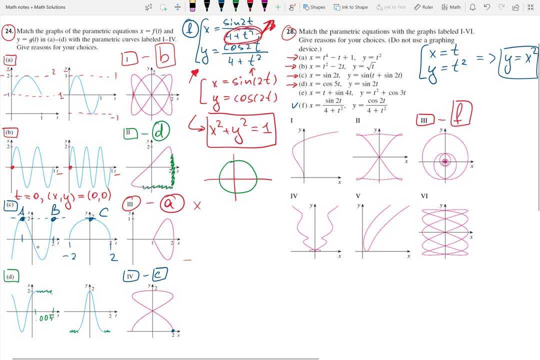 But what if I will return my sine and cosine? It means when my t changes, my parabola is going to increase. The value of my parabola is going to increase, decrease, increase, decrease. And then I need to find the function that looks approximately like a parabola.